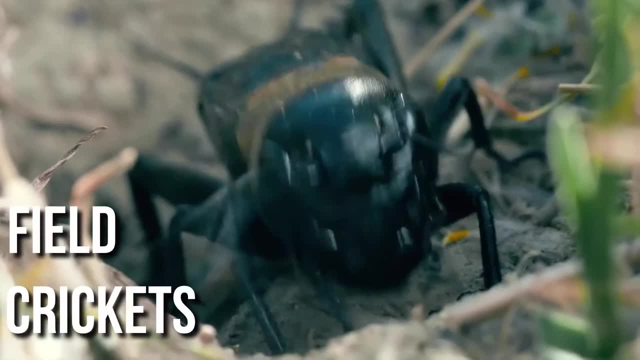 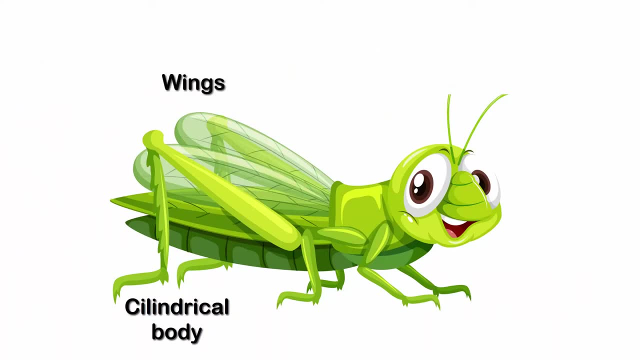 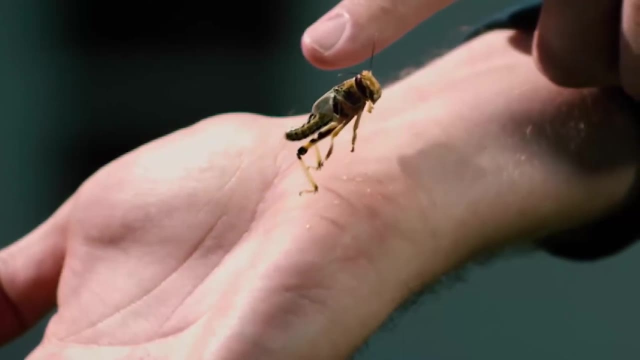 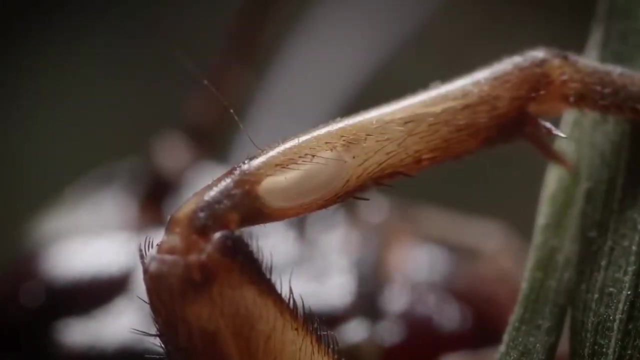 What's about the field crickets? Here are some facts that will help you to know them better. They have cylindrical body wings, a round head and long antennas. The femora of their back legs are greatly enlarged for power jumping. They have the ears in their front legs, so they are very sensitive to vibrations and noises. 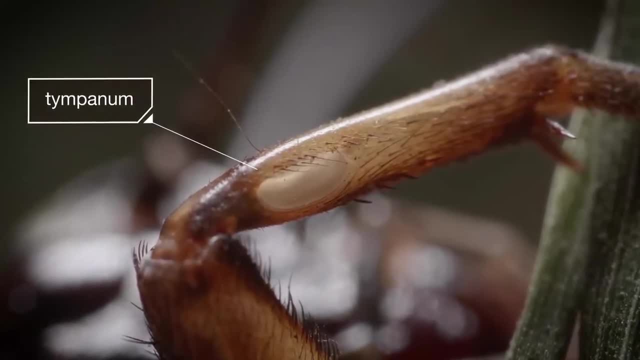 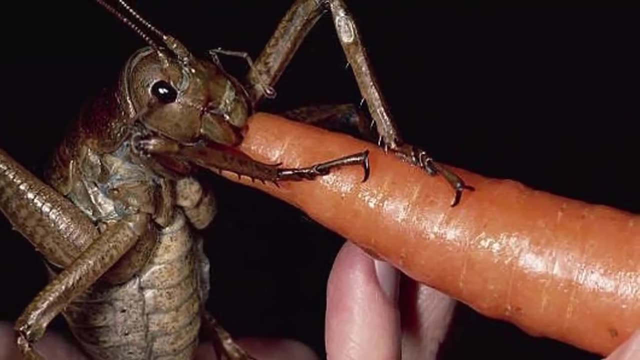 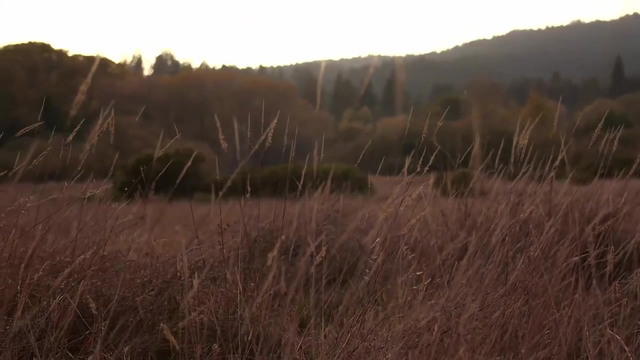 which allows them to find each other and also to avoid possible threats. They are omnivorous: they eat plants, roots, seeds and sometimes other insects and even other crickets. As you may have heard, especially after sunset or at night, they are wonderful musicians. 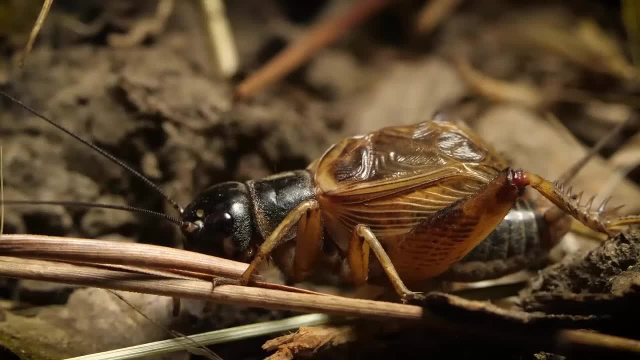 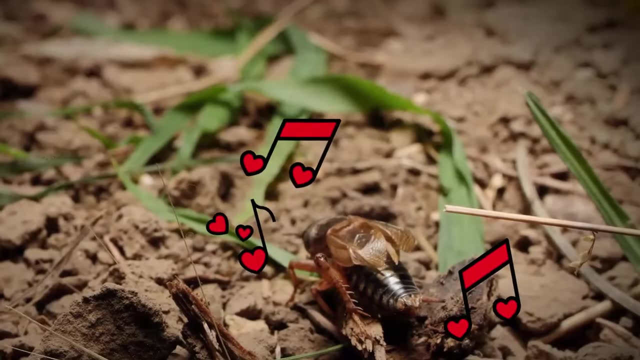 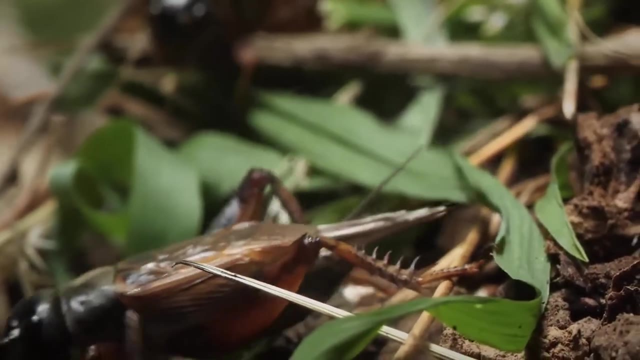 The chirping is produced by stridulating their wings together, but only males do it, And they sing a lovely song For calling their future partner. Well, not always is it a love song. Sometimes can be a fight or war song if another male is around. 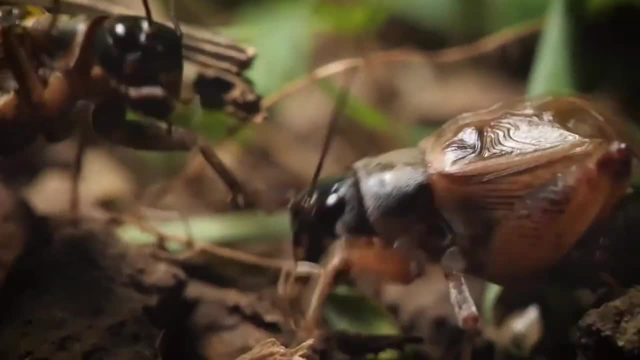 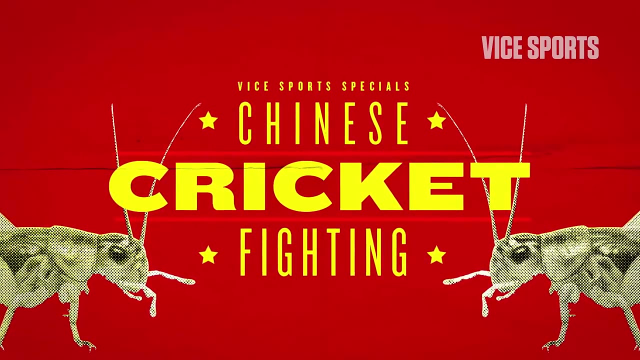 As being territorial is a characteristic behavior of them. In fact, in China, cricket fighting is an old gambling activity. Unlike other fightings, this one rarely causes injuries to the animals And they are usually killed by the crickets. And they are usually killed by the crickets. And they are usually killed by the crickets. Crickets are usually released into the wild after the fighting season ends in later November. Cricket culture in China has a history of 2000 years, and they were also re-birthed. They have regarded a cricket chirpy around the house as an auspicious symbol. 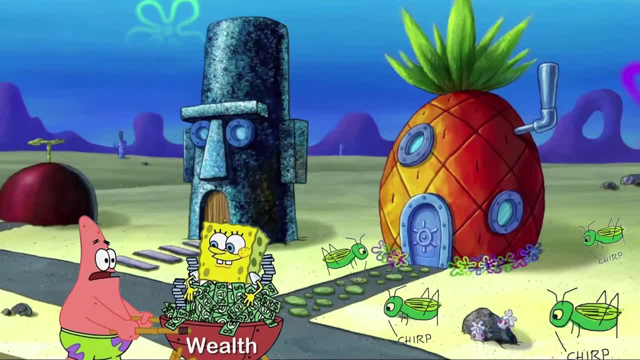 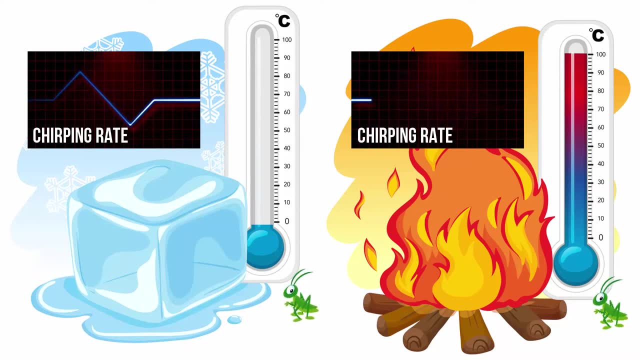 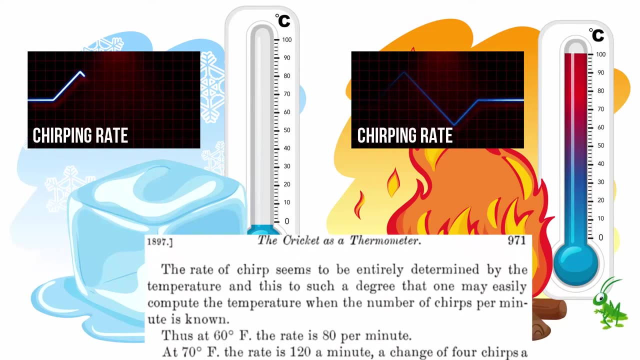 Then cricketing house means wealth will come to the family. But what they really are telling you while they are singing is temperature. Crickets are live thermometers. You can easily calculate the temperature, knowing their chirp rate. This was written in 1897 in an article written by 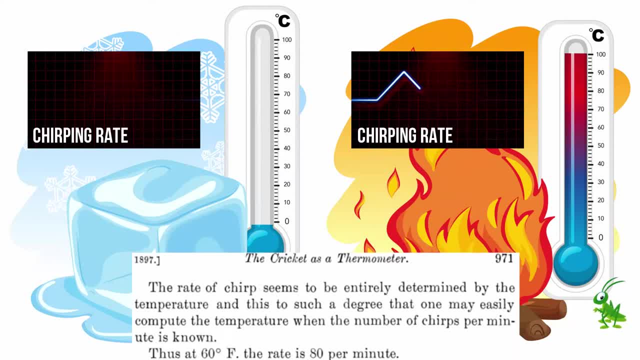 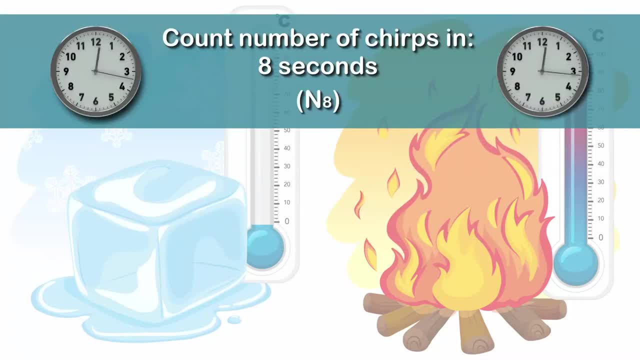 Almos Dolbear, and it is nowadays known as Dolbear's law. The formula is now on screen, but the simplified way would be counting the number of chirps in 8 seconds and adding 5.. That's the surrounding temperature. This seems as: 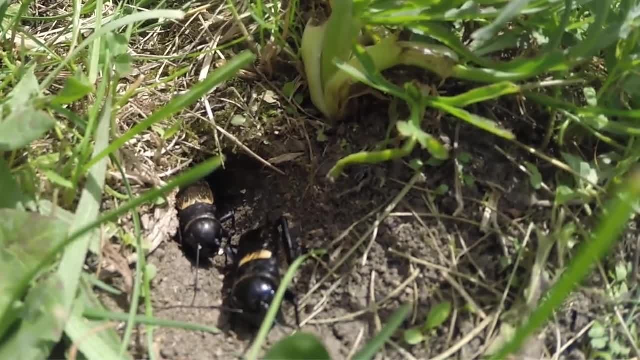 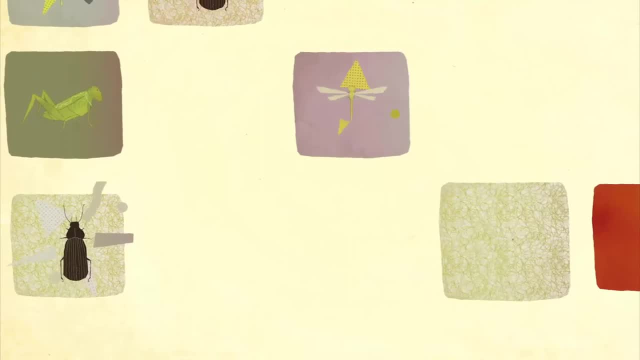 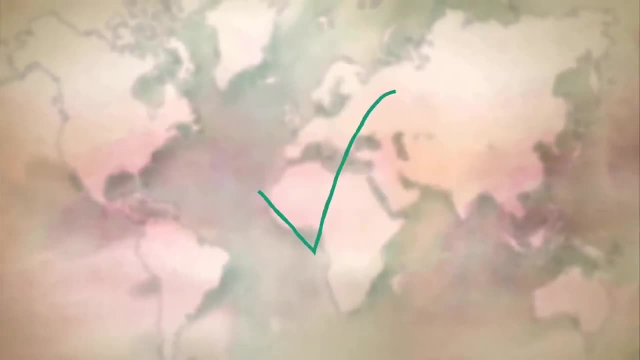 very useful insects, so why don't we give them even more use? They are also edible and very, very nutritious, And although currently in Europe we are not used to eat insects yet, in a lot of places of the world they include them in their weekly diet, And cricket farms consume much less resources than cow or chicken.